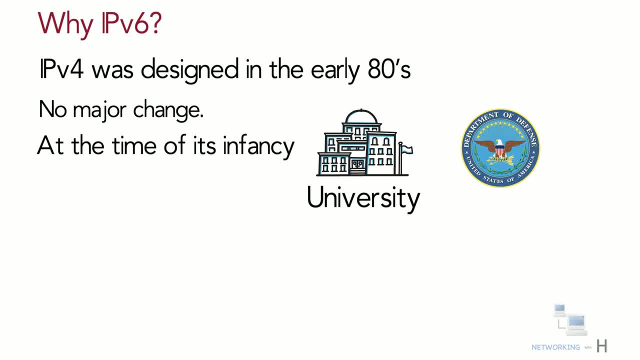 Defense. The Internet Engineering Task Force designed the old IPv4 in 1981 to allow about 4.3 billion addresses, which seemed a lot at that time. Today the number of connected devices in the world far outstrips the available IPv4 addresses. So internet and mobile access now depends on 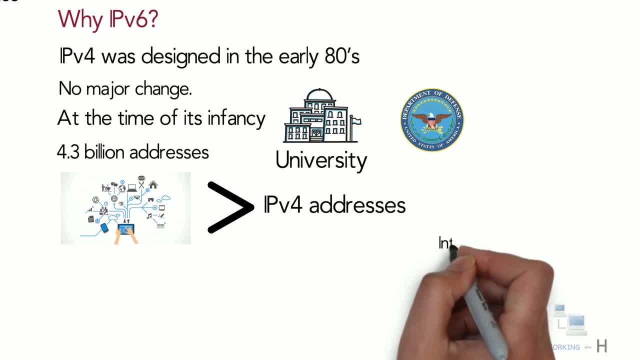 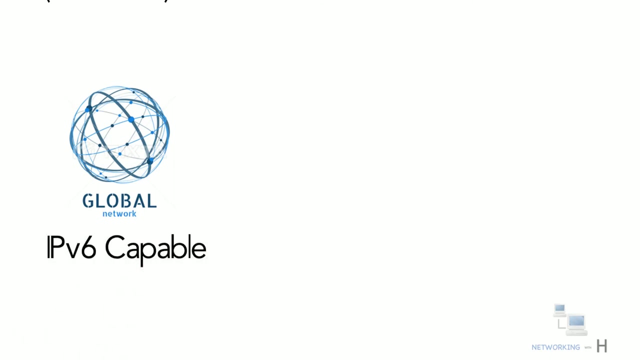 expensive stopgap measures. But as the internet exploded in size and importance, the IETF realized this address limit was looming disaster and designed IPv6.. IPv6 increases the limit to a gigantic 340 undecillion below. Most global networks are already IPv6 capable, but many smaller enterprises and users still need to. 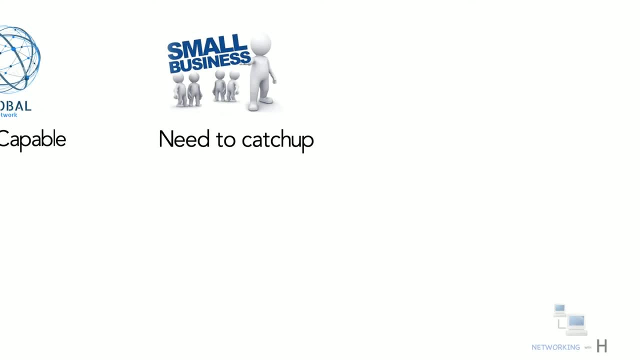 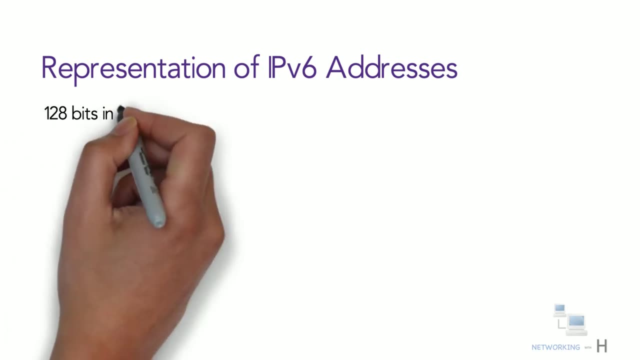 catch up in order to benefit from IPv6.. Let's see how we can represent the IPv6 address. IPv6 addresses are 128 bits in length And uses a convenient hexadecimal or hex format for addresses. In case if you are not aware what hex values are, this table can help you. 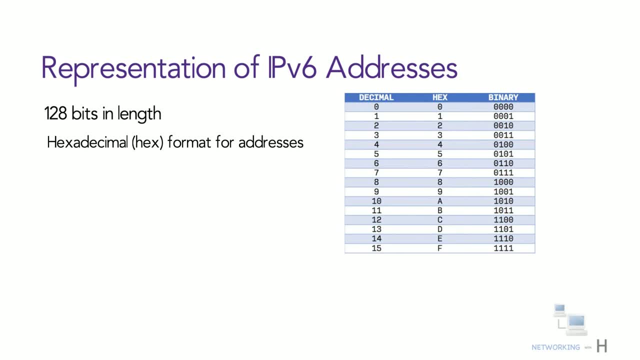 0 to 9 decimal will be represented as 0 to 9 in hex values, And from 10 to 15 in decimal will be represented as A to F, As described in RFC 4291,. the preferred format of IPv6 is 8x. 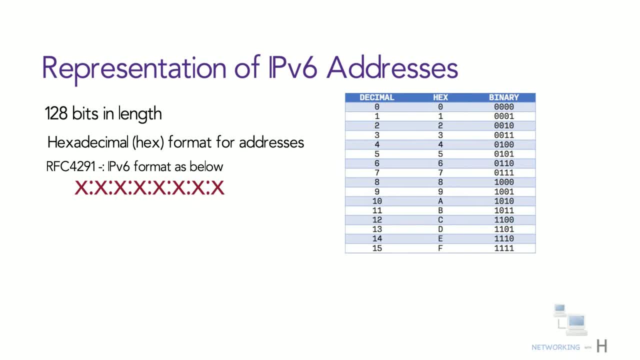 separated by colons. Each x is a 16-bit section that can be represented using up to 4 hexadecimal digits, with the section separated by colons To make it more readable. IPv6 uses a format with 8 sets of 4 hex digits, with each set of 4 digits. 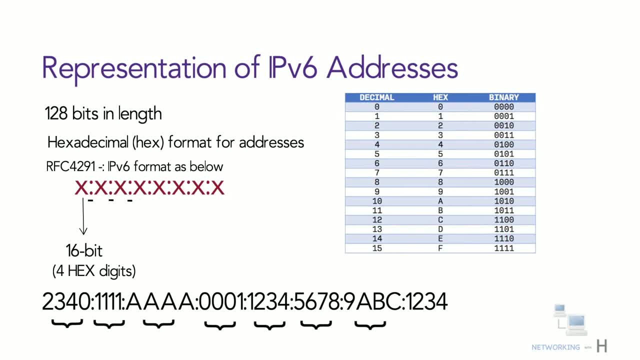 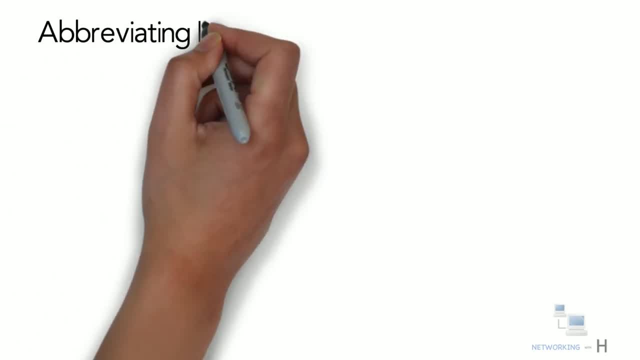 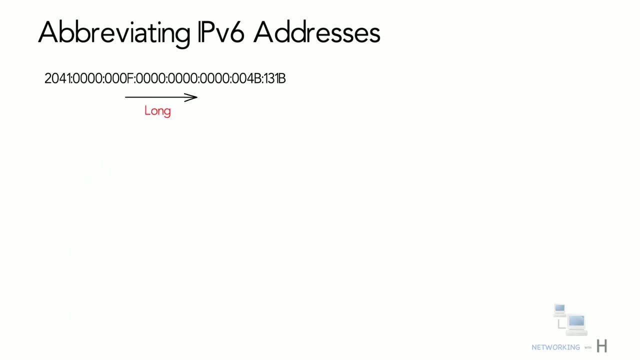 separated by a colon, for a total of 32 hexadecimal values. Next let's see how we can abbreviate the IPv6 addresses. IPv6 addresses are quite long. Imagine you have to call a friend and ask him or her to ping the following addresses: 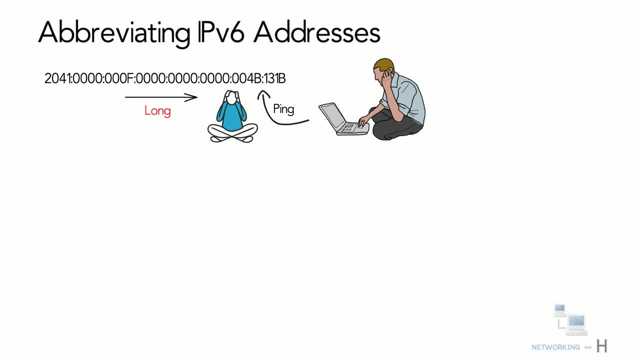 It won't be easy. right To make our lives a bit better, IPv6 addresses can be shortened. You need to just follow the three rules. Rule number one: omit leading zeros. Rule number two: omit all zeros, hexed. Rule number three: four consecutive zeros can be replaced by a single zero. 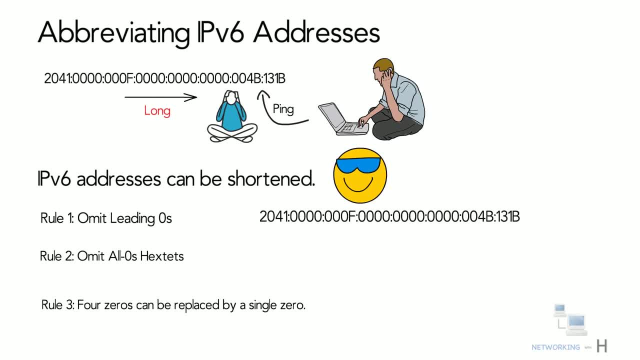 Let us use the above address and apply the rules. First, leading zeros can be removed. Rule number four: After removing the leading zeros, apply the second rule, that is, an entire string of zeros can be removed and replaced by a double colon. 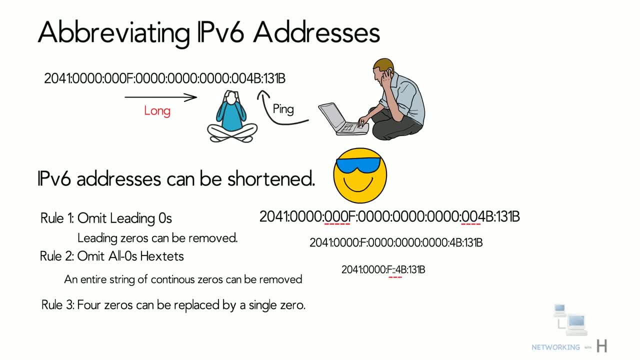 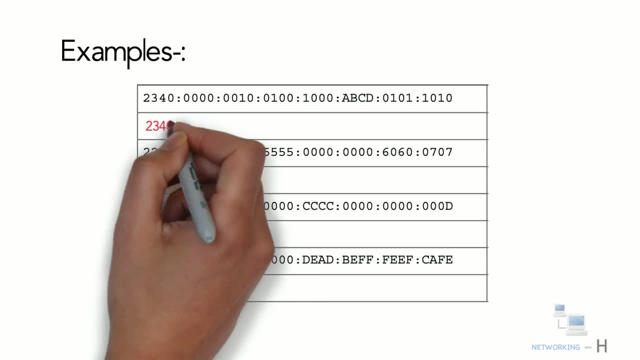 You can do it only once. Then you can apply rule number three, where four consecutive zeros can be replaced by a single zero. Let's take a look at some of the examples, where I'll show you the original IPv6 and followed by short abbreviated addresses. 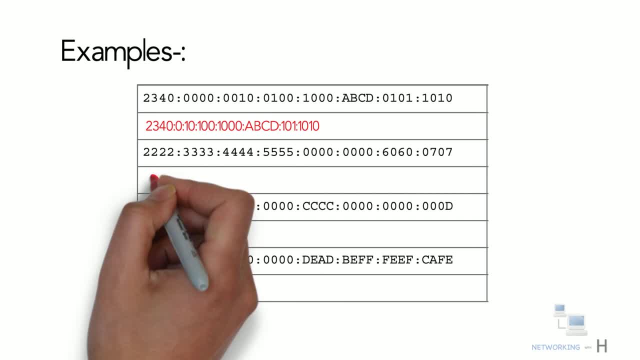 Let's take a look at some of the examples where I'll show you the original IPv6 and followed by short abbreviated addresses. Let's take a look at some of the examples where I'll show you the original IPv6 and followed by short abbreviated addresses. 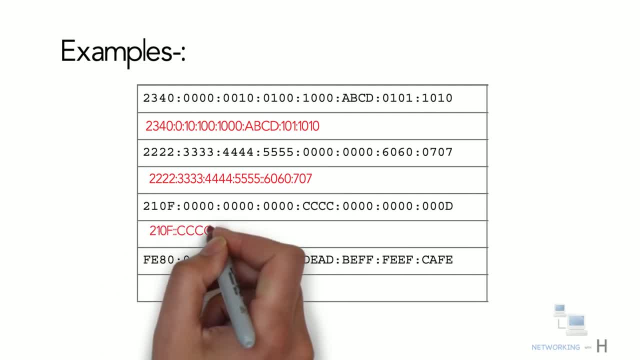 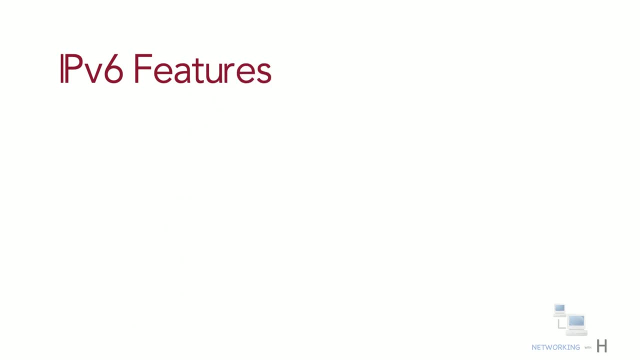 The consecutive zeros are removed. The consecutive zeros are removed Here. the consecutive zeros are removed as well. Next, let's look at the IPv6 features, Starting with larger address space. In contrast to IPv4. IPv6 uses 4 times more bits to address a device on the internet. 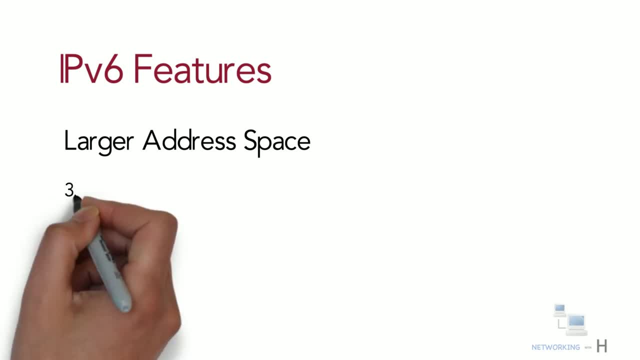 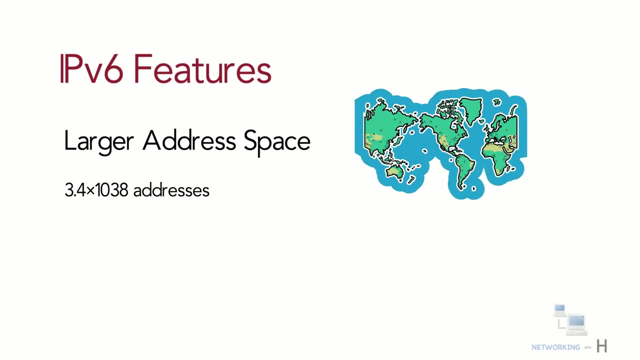 This much of extra bits can provide approximately 3.4 x 10-38 different combination of addresses. This address can accumulate the aggressive requirement of address allotment for almost everything in this world. According to an estimate, 1564 addresses can be allocated to every square meter of this. 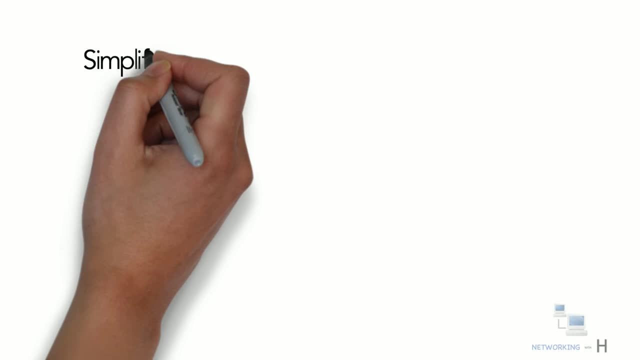 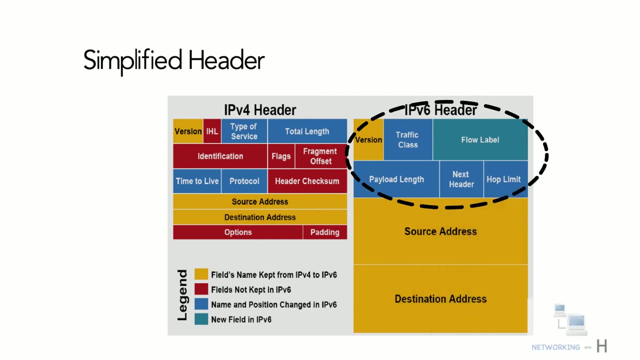 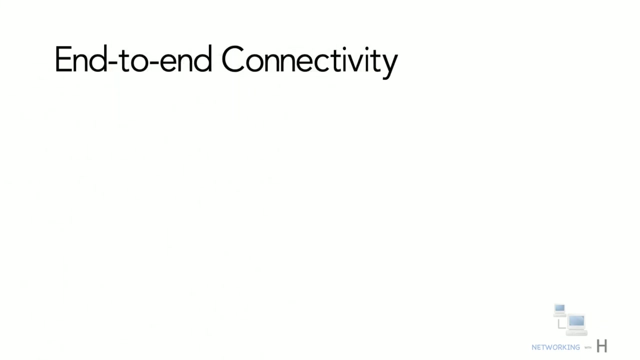 earth. The next feature we have is Simplified header. IPv6 header has been simplified by moving all unnecessary information and options which are present in IPv4 header. The next feature we have is end-to-end connectivity. Every system now has unique IP address and can traverse through the internet without 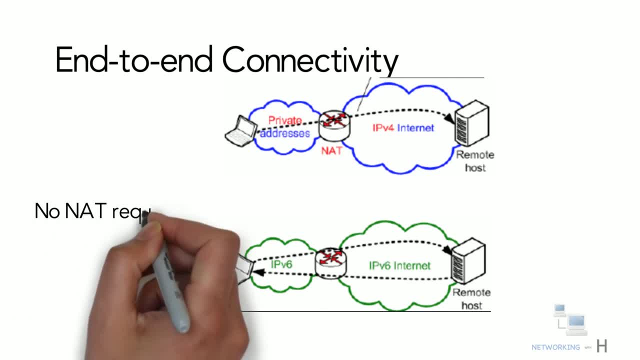 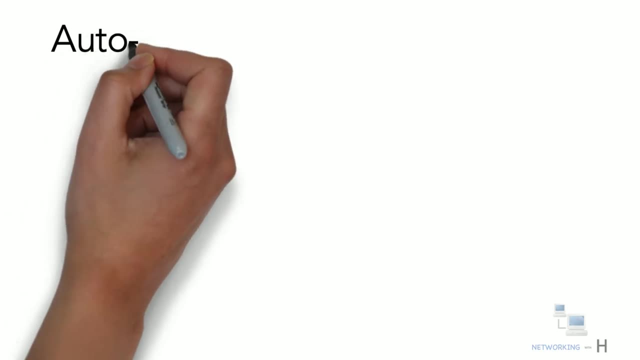 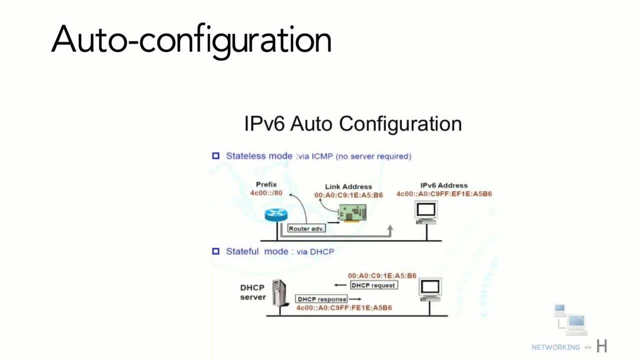 using network address transfer. Obviously, if we would necessarily like, we won't need it, for��he end��터 doesn't make these issues. The next feature we have is Auto-Configuration. IPv6 supports both stateful and stateless auto-configuration mode of its host devices. 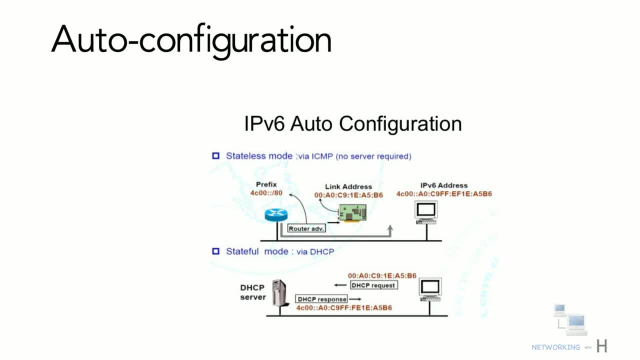 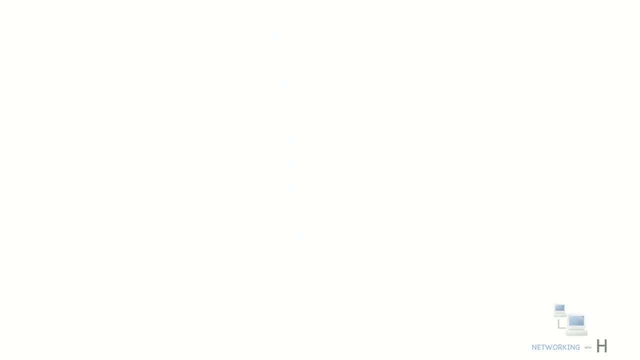 This way, absence of holidays of DACP server does not put a halt on inter-segment communication such as IDC şポ promotıca şiddet og IPv6 pers. comparison to IPv2. Android UI evaluations- Sub unchecked. The next feature we have is faster forwarding or routing. 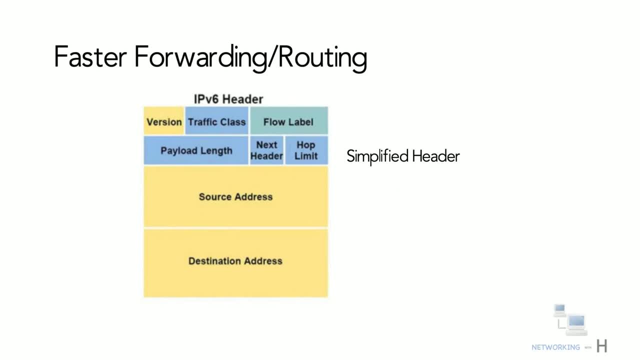 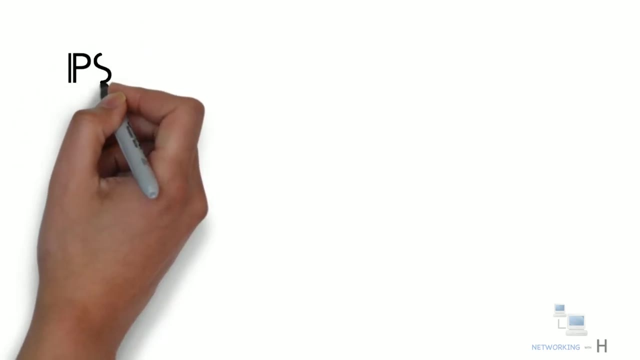 Simplified header puts all unnecessary information at the end of the header. The information contained in the first part of the header is adequate for a router to take routing decisions, thus making the routing decision as quickly as looking at the mandatory header. The next feature we have is IPsec. 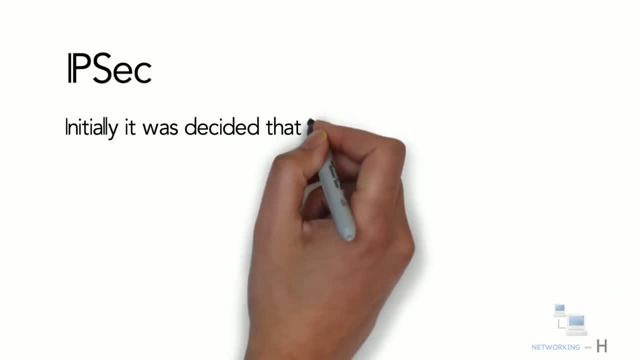 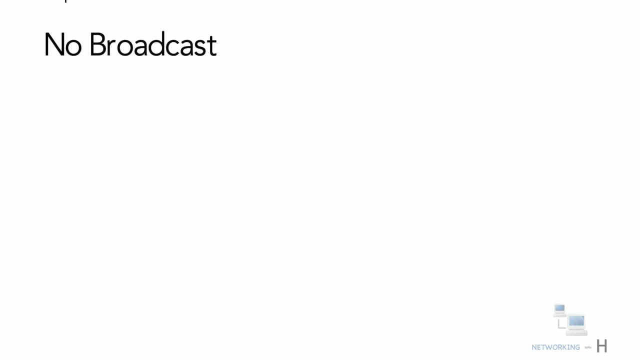 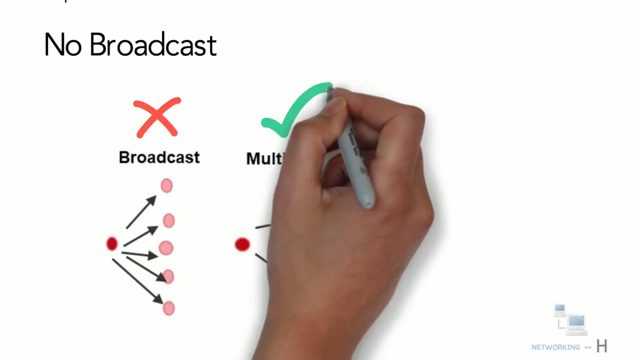 Initially, it was decided that IPv6 must have IPsec security, making it more secure than IPv4.. This feature has now been made optional. Another feature we have is no broadcast. IPv6 does not have any broadcast support anymore. It uses multicast to communicate with multiple hosts. 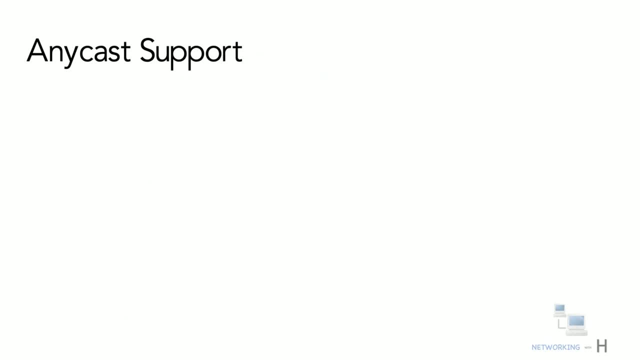 Another important feature is anycast support. This is another characteristic of IPv6.. IPv6 has introduced anycast mode of packet routing. In this mode, multiple interfaces over the internet are assigned same anycast IP address. Routers, while routing, send the packet to the nearest destination. 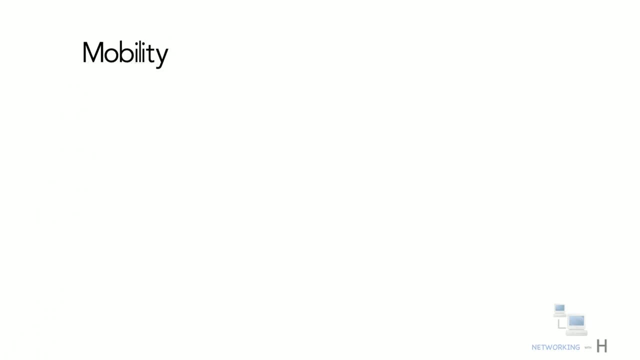 Another feature we have is mobility. IPv6 was designed keeping mobility in mind. This feature helps. This feature enables hosts, such as mobile phones, to communicate with each other. This feature helps. This feature enables hosts, such as mobile phones, to communicate.